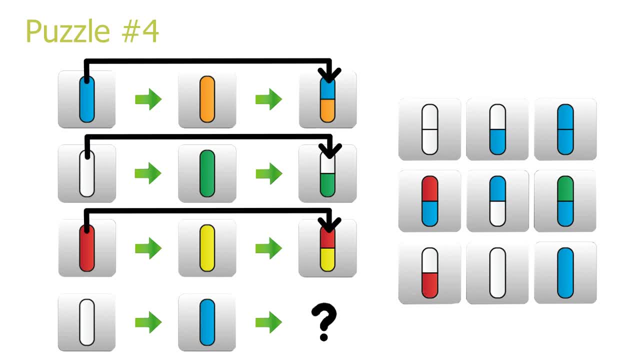 Puzzle number 4.. The third picture in a row has the top half color of the first picture and the bottom half color of the second picture. Looking at the fourth row, we have a white top half and a blue bottom half. Answer 2 is the correct solution. Puzzle number 5.. 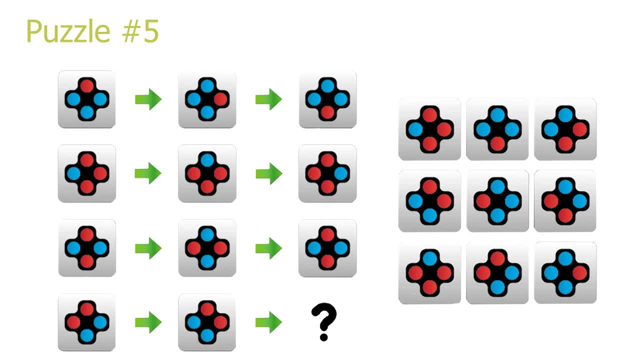 This is a puzzle with rotation in the rows. Moving from the first picture in a row to the second picture, we have a 90° clockwise rotation, And moving from the second picture to the third picture, we have another 90° clockwise rotation. To solve the puzzle we 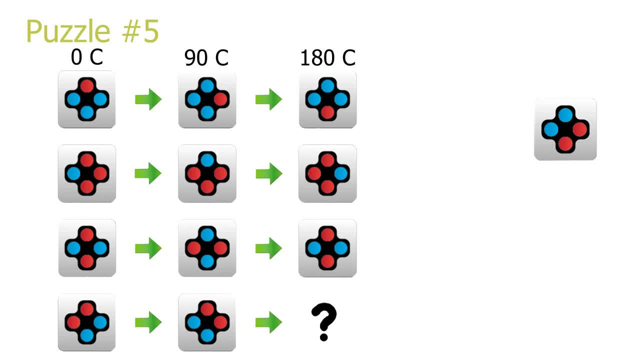 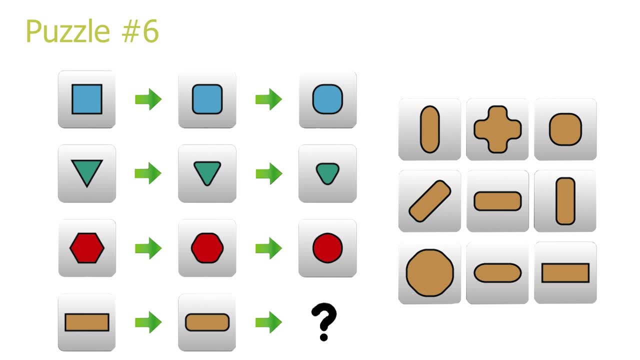 go by the fourth row and we rotate the second picture by 90° clockwise. This gives answer 3 as the correct solution. Puzzle number 6.. In this puzzle we have a smoothening of the edges To solve the puzzle. the first thing to notice is that the general rotation and shape is conserved. This leaves 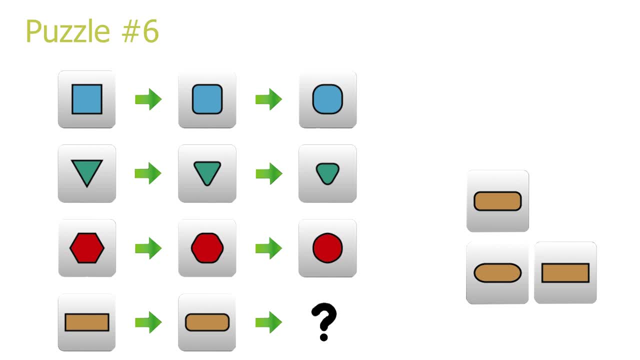 Either answer 5,, 8 or 9 as the correct answer. If we look at the second picture in the fourth row, our answer has to be more smooth than that picture. Answer 5 is identical to the second picture and therefore not correct. 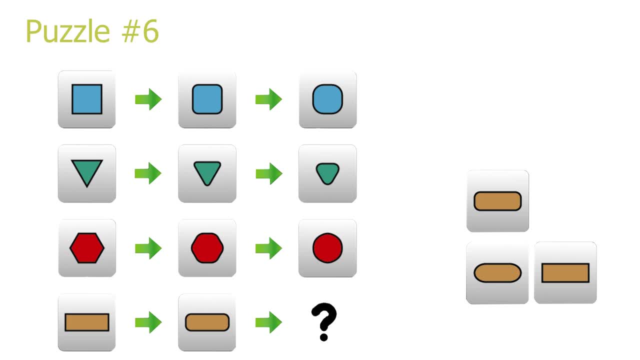 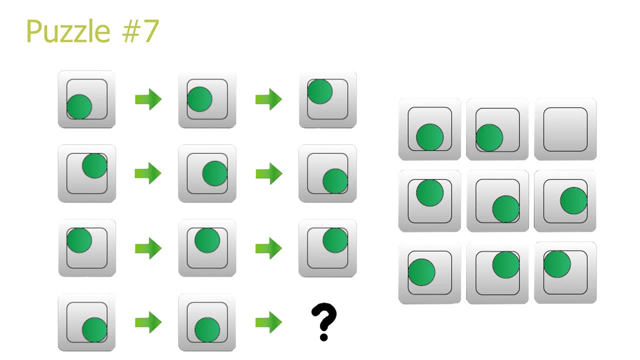 And answer 9 is less smooth than the second picture and therefore not correct. This leaves answer 8 as the correct solution. Puzzle number 7.. I think the easiest way to explain this puzzle is by using the first row as an example. Notice that the position of the circles in each picture can be described by a dot in. 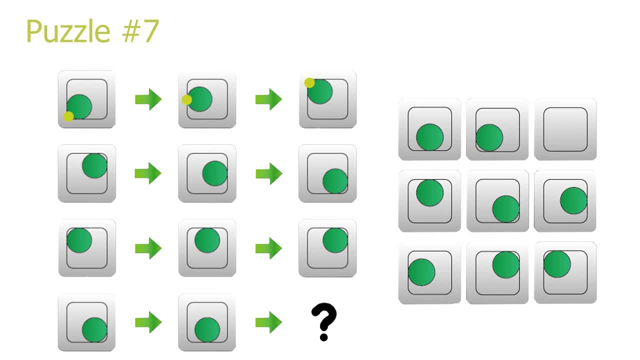 the bottom left corner, a dot in the middle left and a dot in the top left corner. In total, we have 8 of these dot positions and, moving to the right in a row, the circle always moves to the next dot in a clockwise direction. 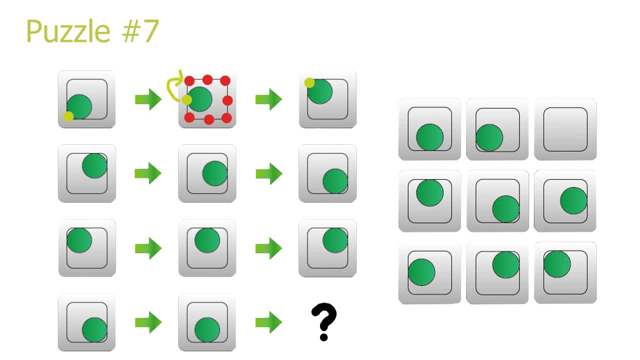 To solve the puzzle we look at the fourth row. The second picture has a circle in the bottom middle and moving it once in a clockwise position will lead to a circle in the bottom left corner. Answer 2 is the correct solution. Puzzle number 8.. 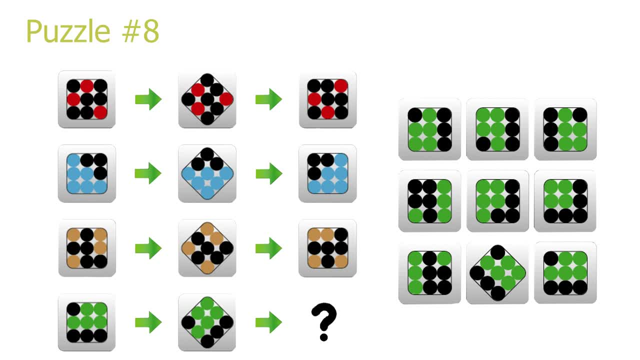 Another rotation puzzle. Moving from the first to the second picture in a row, we have a 45 degree counterclockwise rotation, And moving from the second to the third picture, we have another 45 degrees counterclockwise rotation. Going by the fourth row and doing the rotation, we get answer 2 as the correct solution. 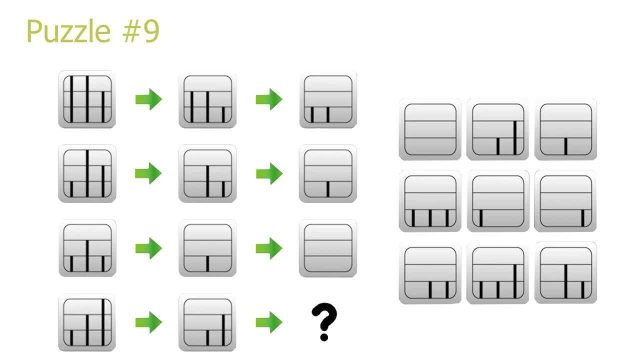 Puzzle number 9.. This is a row puzzle where we reduce the height of the lines by one as we move to the right in a row. I will show you in the first row how I see this puzzle in my head. Looking at the first picture, we get the bottom portion chopped off and it falls down to create 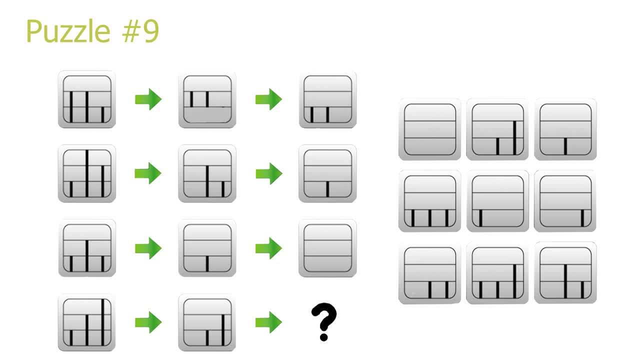 the second picture. Looking at the second picture, we get the bottom portion chopped off and it falls down to create the second picture. Looking at the third picture: To solve the puzzle, we just do the same thing for the second picture in the fourth row. 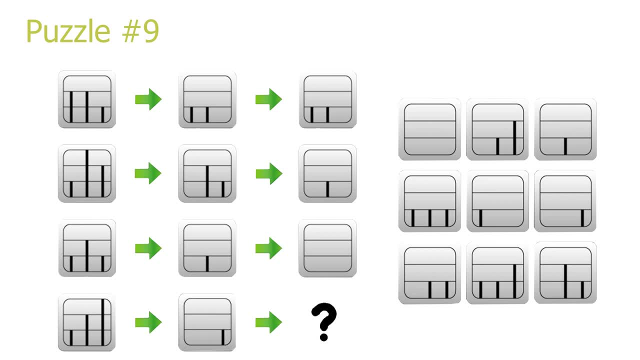 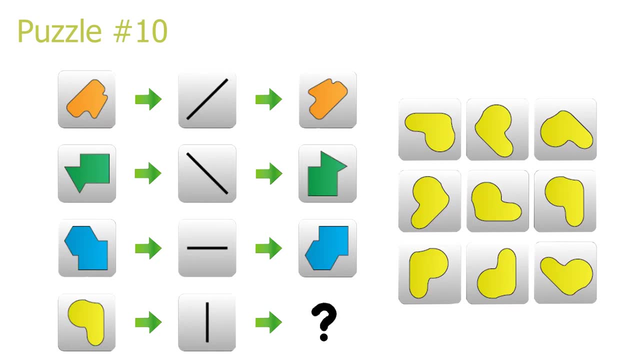 We chop off the bottom portion and it falls down. This is identical to answer 6.. Answer 6 is the correct solution. Puzzle number 10.. This is a mirroring puzzle. The pictures in the second column give this line of mirroring. 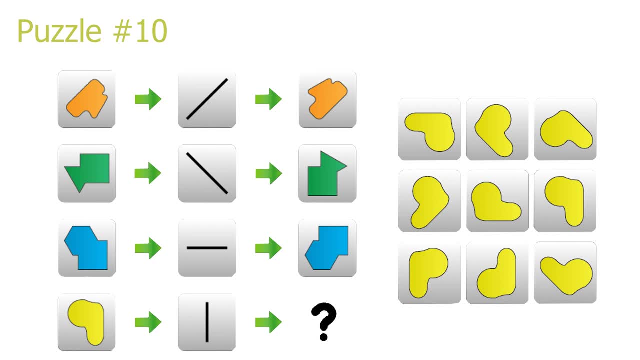 And the pictures in the first column is mirrored by this line to create the pictures in the third column. Personally, I dislike visualizing this mirroring effect. Instead, I picture a pancake and a spatula. The pictures in the first and the third column are mirrored by this line to create the pictures. 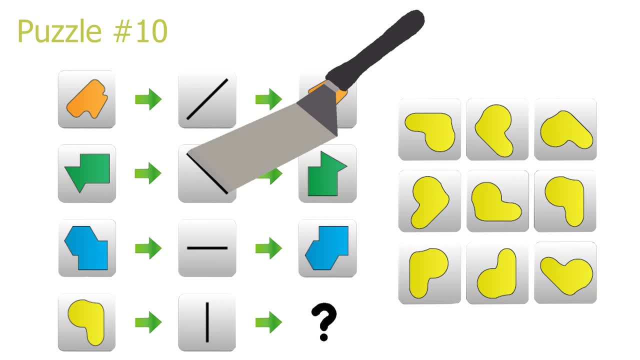 and the third column are these weirdly shaped pancakes, And the tip of the spatula is shown by the line of mirroring in the second column. To produce the third picture in a row, we simply flip the first picture in the row forwards or backwards compared to the tip of the spatula. 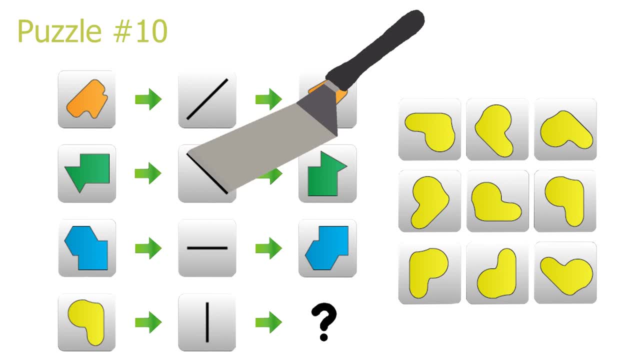 This flipping is perfectly 180 degrees and lines back on the pan. To solve the puzzle, we just flip the first picture in the fourth row directly to the left or the right. This gives answer 7.. Answer 7 is the correct solution. 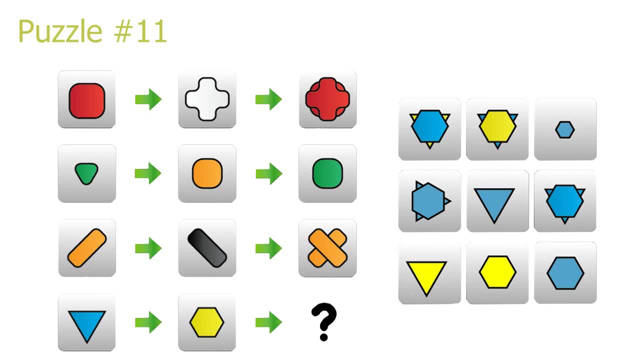 Puzzle 11.. In this puzzle, to create the third picture in a row, we just flip the first picture in the fourth row, We take the second picture in the row and turn it the same color as the first picture, and then we place the second picture on top of the first picture. 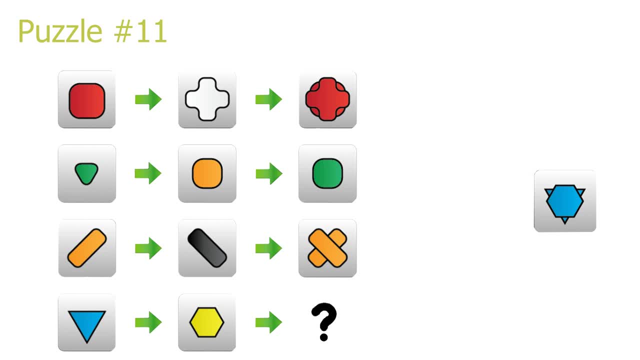 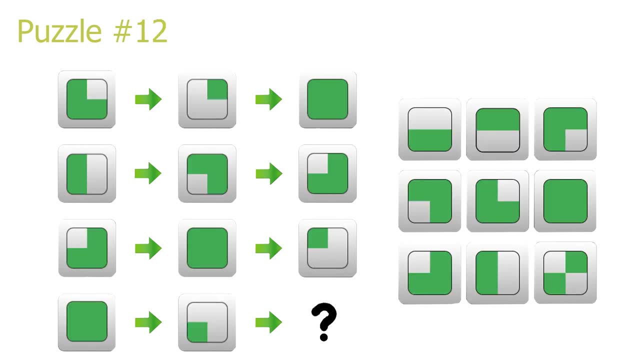 To solve the puzzle, we do this for the fourth row and we get a blue hexagon on top of a blue upside down triangle. Answer 6 is the correct answer. Puzzle 12.. This is an addition puzzle with cancellation. To produce the third picture in a row, we add the first and the second picture with. 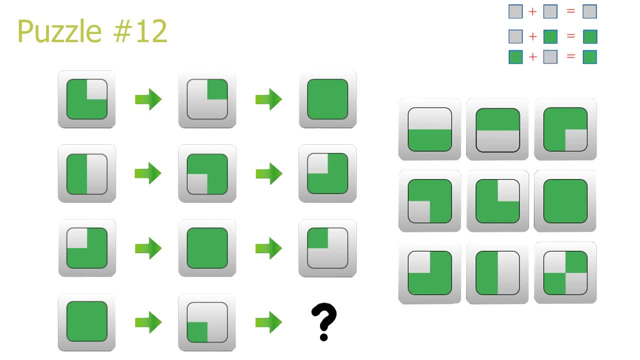 the following rules: Gray plus gray equals gray, Gray plus green or green plus gray equals green, And green plus green equals gray. To solve the puzzle, we follow these rules for the fourth row and we get a gray area in the bottom left corner and the rest of the corners are green. 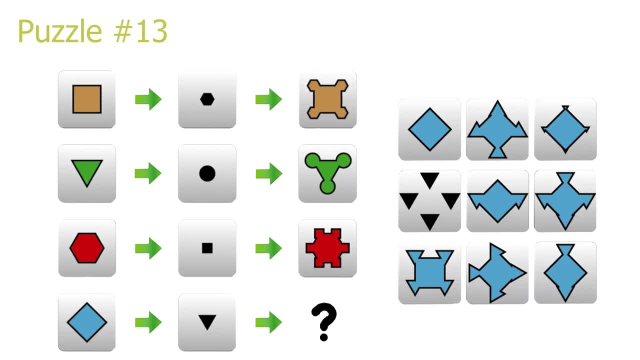 Answer 4 is the correct solution. Puzzle 13.. In this puzzle we have polygons in the first column and even smaller polygons in the second column. To produce the third picture in a row, we place the second picture in each of the corners. 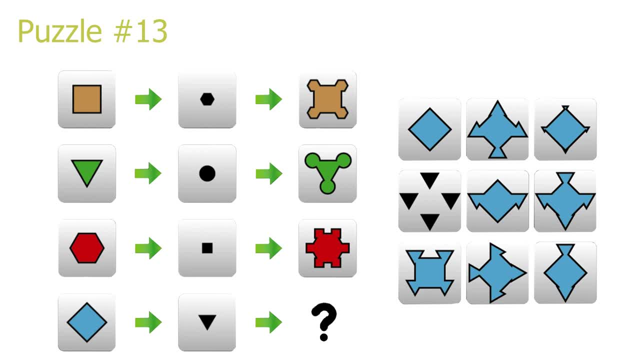 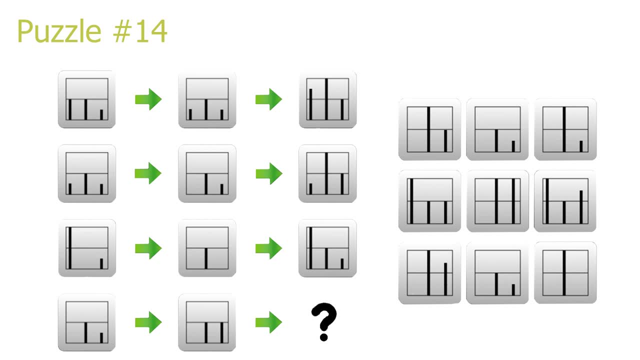 of the polygon in the first picture and then turn them the same color as the first picture, Doing this for the fourth row, we get answer 6 as the correct solution. Puzzle 14.. This is a simple addition puzzle. To get the third picture in a row, we add the height of the black lines in the two first. 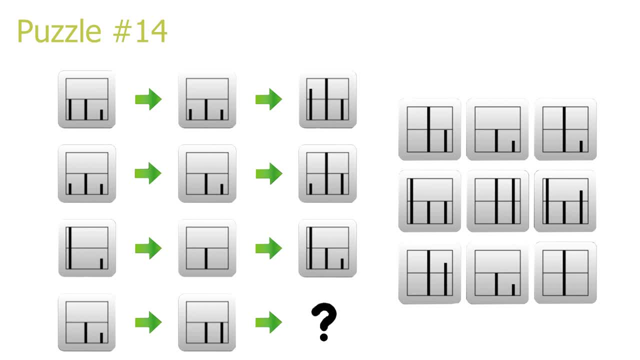 pictures. To solve the puzzle. we go by the fourth row. The left side is 0 plus 0, equaling 0 height, The middle is 2 plus 2, equaling 4 height, And the right is 1 plus 2, equaling 3 height. 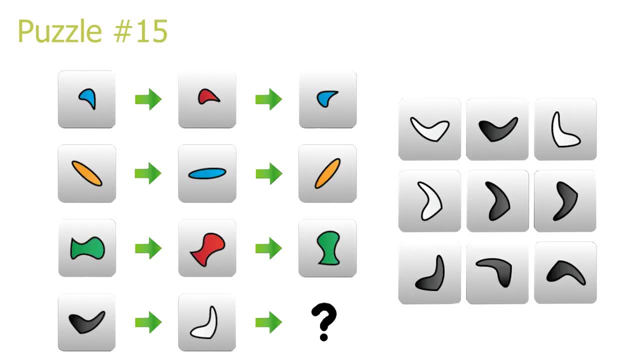 Answer 7 is the correct solution. Puzzle 15.. This is a rotation puzzle. Going from the first to the second picture in a row, we have a 45 degree counterclockwise rotation. Then, going from the second to the third picture, we have another 45 degree counterclockwise. 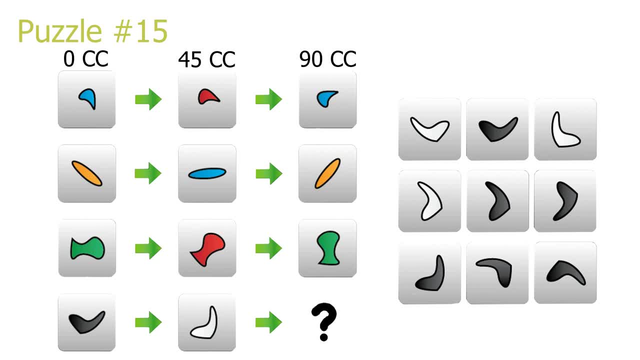 rotation. There is also a color component to the puzzle, where the first and the third picture in a row have the same color. Going by the fourth row and rotating the first picture by 90 degrees counterclockwise or the second picture by 45 degrees counterclockwise, we get answer 5 as the correct solution. 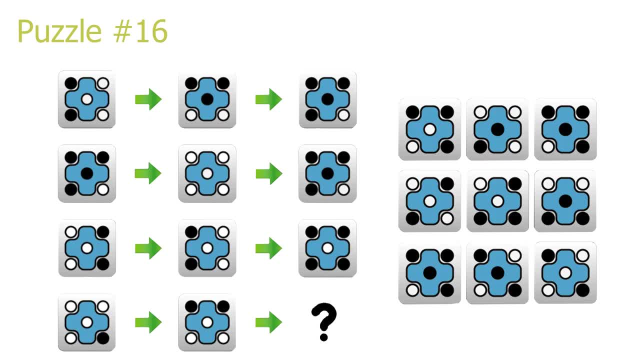 Puzzle 16.. In this puzzle we simply add the first and the second picture to produce the third. We have these five circles which are either black or white. If the circles are black in either one or both the first pictures, then the circle will. 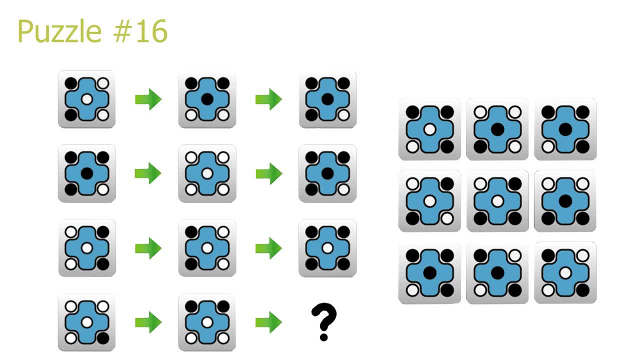 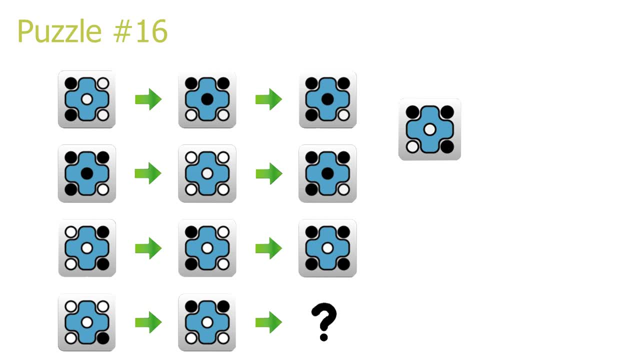 be black in the third picture. To solve the puzzle we go by the fourth row. We get a black circle in the bottom right corner, in the top left corner and in the top right corner. Answer 1 is the correct solution: Puzzle 17.. 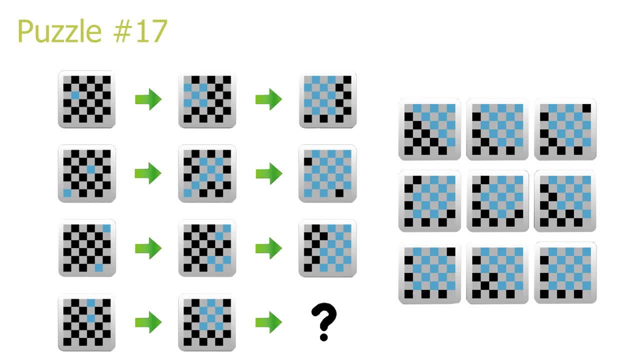 To explain this puzzle, I'm going to use the first row as an example. If we look at the first picture in the first row, we see that the blue squares is next to these four squares, which gets colored blue to produce the second picture. 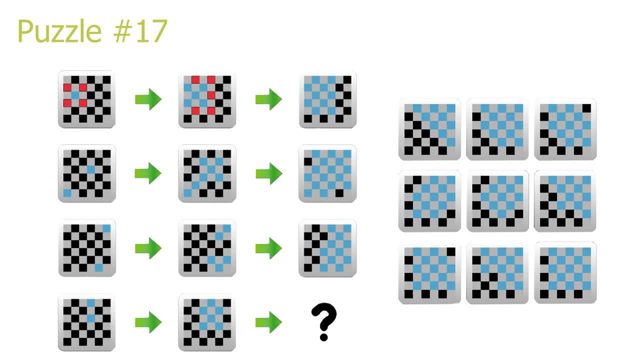 Puzzle 17.. In the first picture we have these five black squares next to the blue squares, which again gets colored blue to produce the third picture. To solve the puzzle, let's look at the fourth row. In the first picture we have these four black squares next to the blue squares and in the 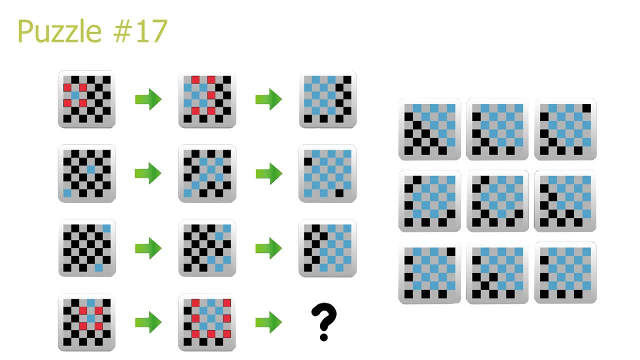 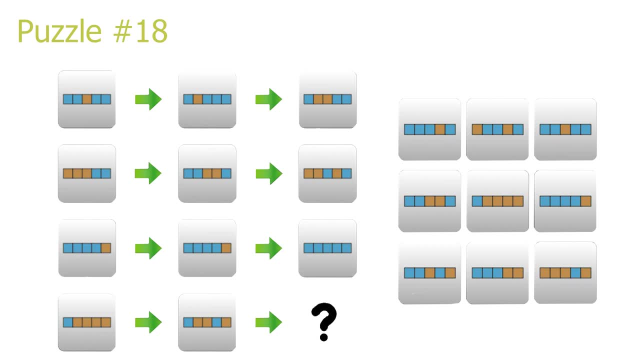 second picture we have these seven black squares next to the blue squares. Turning these blue gives answer 9 as the correct solution. Puzzle 18.. This is an addition puzzle with cancellation, with the following rules: Blue plus blue equals blue, blue plus orange or orange plus blue equals orange and orange. 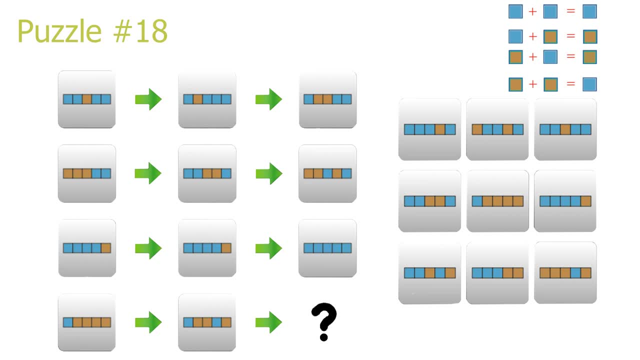 plus orange equals blue. To solve the puzzle, we follow these rules for the fourth row. This gives an orange square in the fourth slot and the rest are blue. Answer 1 is the correct solution: Puzzle 19.. I personally struggled to find some clear rule to solve this puzzle at first. 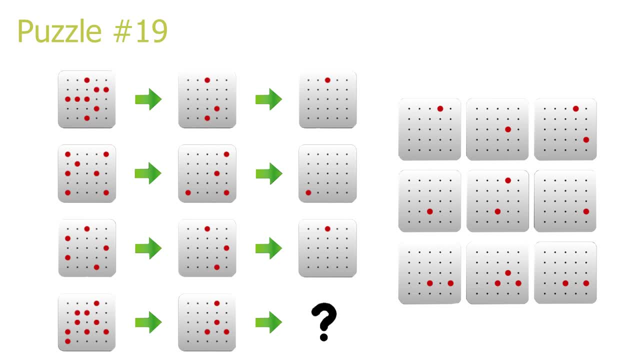 I think it's a very interesting puzzle, so if you haven't solved it by yourself yet, I suggest that you pause the video and keep trying to solve it. To explain the puzzle, I'll go quickly through each of the rows. If we look at the first row, the first picture have five dots, which are right next to the. 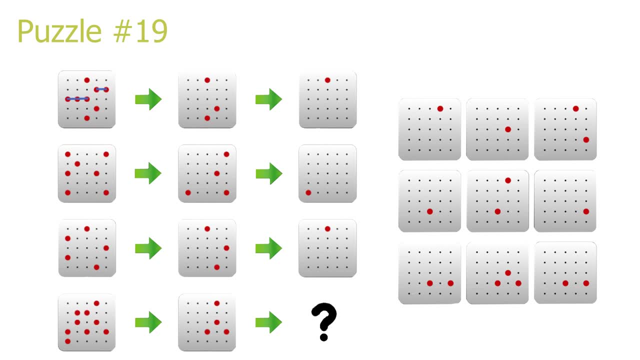 second picture and these five dots are removed to make the second picture. In the second picture, we have these two dots on the bottom, which are removed. Now, what does moving from the first to the second picture and moving from the second to the third picture have in common? 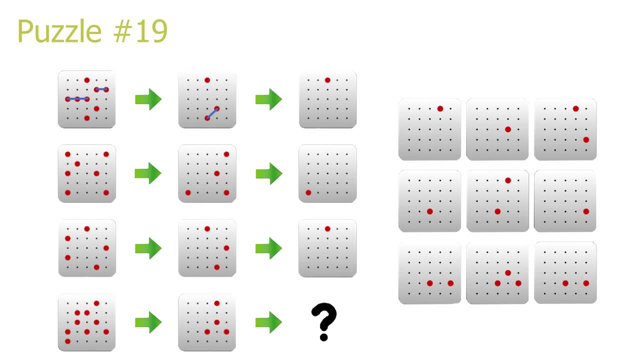 All the dots which have the shortest distance to another dot is removed. It becomes more clear when we go through the next rows: The shortest distance between dots in the first picture, in the second row are these three dots in the top left corner and in the second picture it's these three dots on. 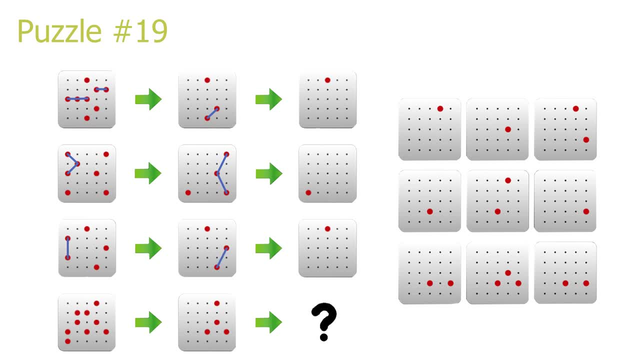 the right side. For the third row, we have two on the left and then two on the bottom right. For the fourth row, we have five on the left side and then three on the right side. Removing these three leads to answer one as the correct solution. 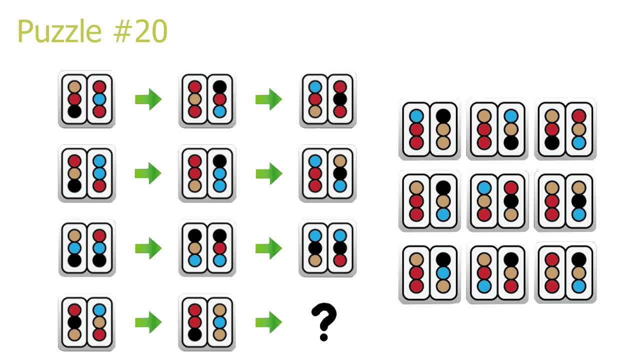 Puzzle number 20.. In this puzzle we have these colored circles which move in some pattern. I'll use the first row as an example. The circles on the left side are always pushed down, and the same holds true for the right side. 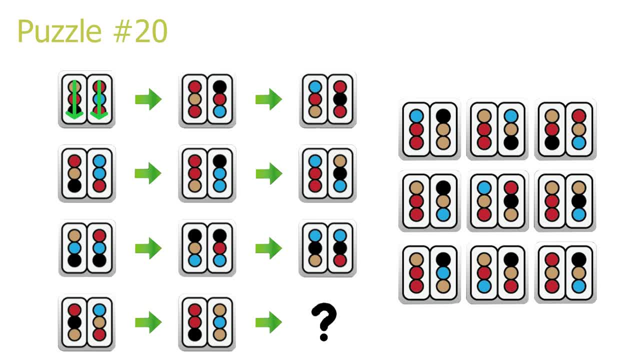 The bottom circles are pushed outside the picture and reappear on the top side. on the opposite side, The circles on the right side reappear on the top right and the bottom right reappear on the top left. To solve the puzzle, we just move the circles like this in the second picture, in the fourth, 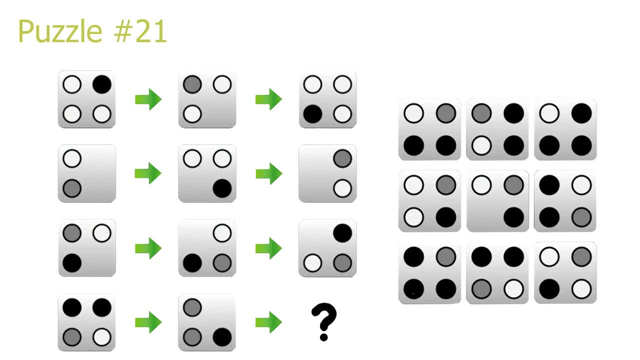 row. This leads to answer four being the correct solution. Puzzle number 21.. In this puzzle, we have four positions and two types of circles. We have black circles and white circles. A gray circle is just a black and a white circle on top of each other. 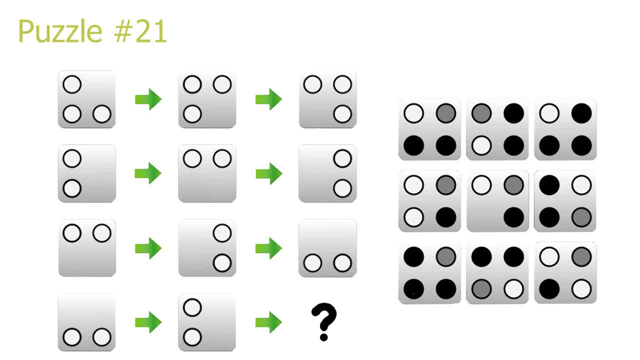 Let's start by focusing only on the white circles. We can quite easily see how moving to the right in a row leads to the white circles moving in one position in a clockwise direction. Looking at the fourth row, we can see that there will be two white circles on the top. 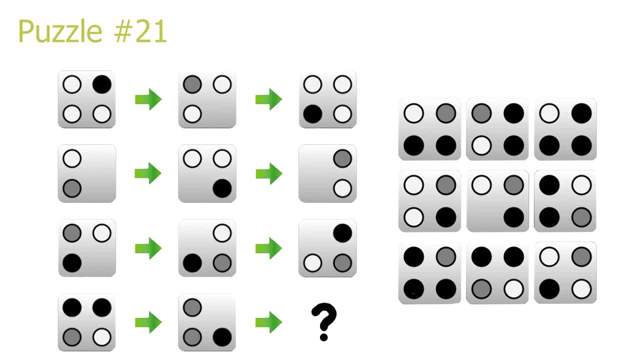 left and top right in our correct answer. Adding the black circles back in, we see that the black circles move in the opposite direction of the white circles. They move in one position in a counterclockwise direction. Looking at the second picture, in the fourth row we can see three black circles and rotating. 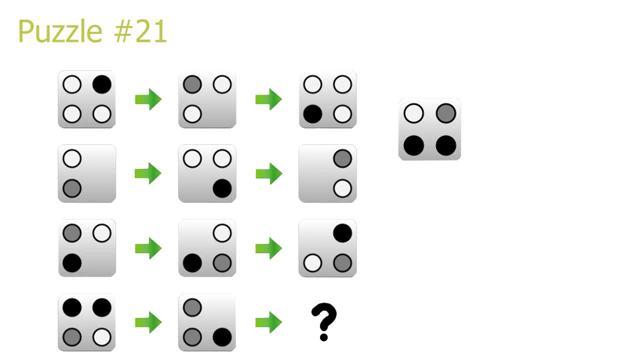 them once in a counterclockwise direction will lead to a black circle in the bottom left and bottom right corner. The black and white circles in the top right corner fuse together into a gray circle And there will be a white circle in the top left corner. 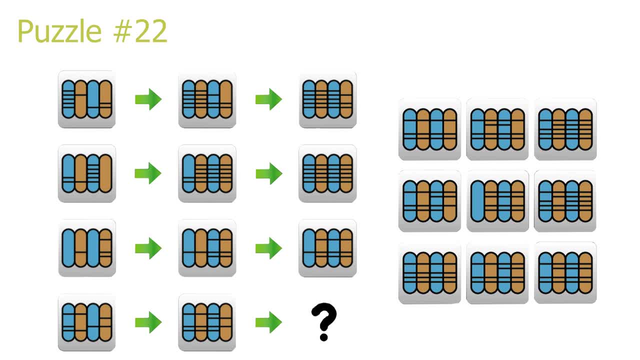 Answer 1 is the correct solution: Puzzle 22.. In this puzzle we have these lines on blue and brown segments. The lines always extend to the neighboring segments. To solve the puzzle, we just look at the fourth row and we see that there will be a full. 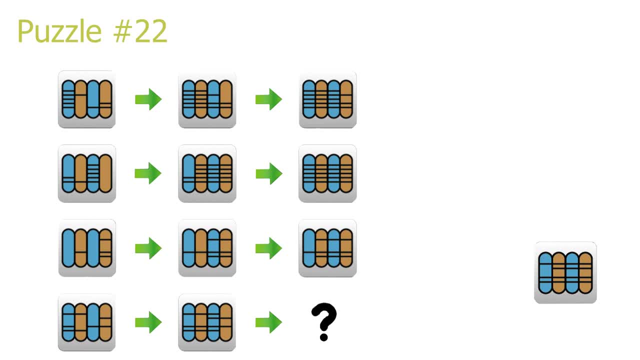 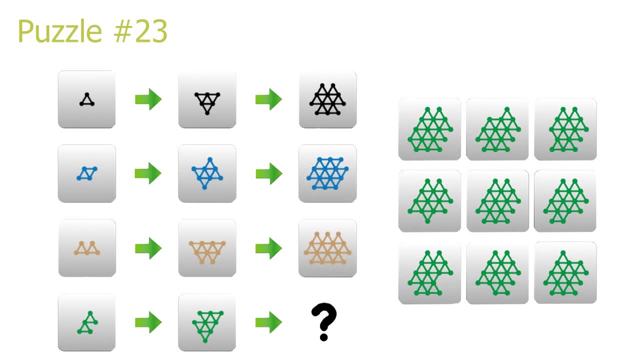 line on top, on the second bottom and on the bottom. There will be no line in the middle and three quarters of a full line on the second top. Answer 9 is the correct solution. Puzzle 23.. In this puzzle we add new triangles on the circle. 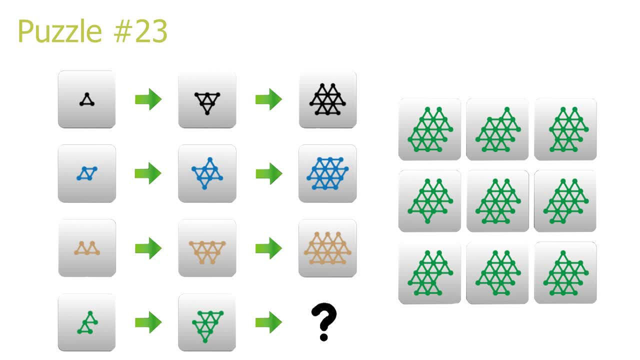 Answer 3.. In this puzzle we add new triangles on the surface of the previous structure. I found this puzzle quite easy because of a shortcut I found First. we can just ignore the two first rows. We see that the pictures in the fourth row is simply the pictures in the third row, rotated. 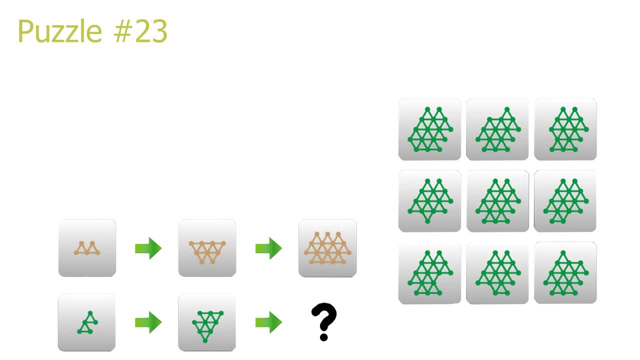 roughly 120 degrees in clockwise direction and turned green. To solve the puzzle, all we do is to rotate the third picture in the third row by roughly 120 degrees in clockwise direction. This leads to answer 5 being the correct solution: Puzzle 24.. 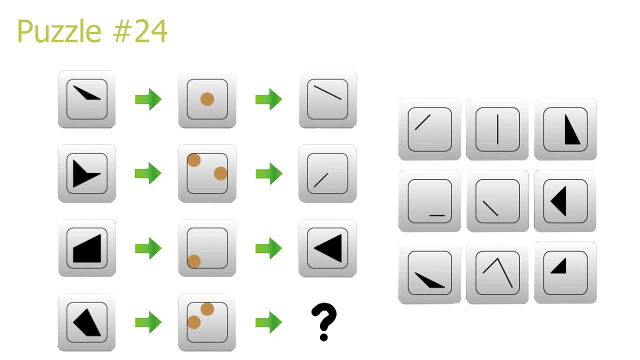 This is a very fun and easy puzzle. The first column have these polygons. The polygons consist of points and lines extended between these points. The circles in the second column indicate which points we should remove in order to create the polygon in the third column. 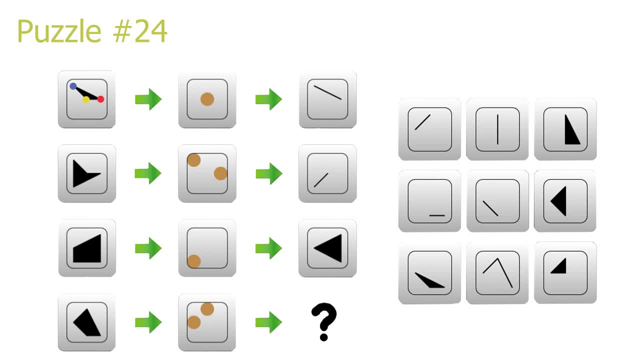 In the first row, for example, the polygon have three corners. The circle in the second picture indicate that we should remove the yellow corner. This leaves only the blue and the red point left, and extending a line between these leads to the third picture. 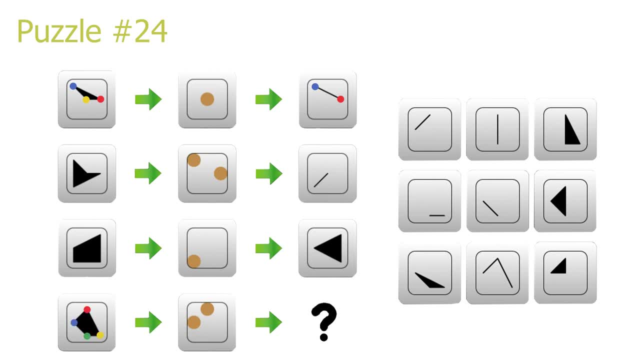 To solve the puzzle we go by the fourth row. The polygon have four points and the second picture indicates that we should remove the red and the blue points. This leaves only a line between the green and the yellow point in our answer. Answer 4 is the correct solution. 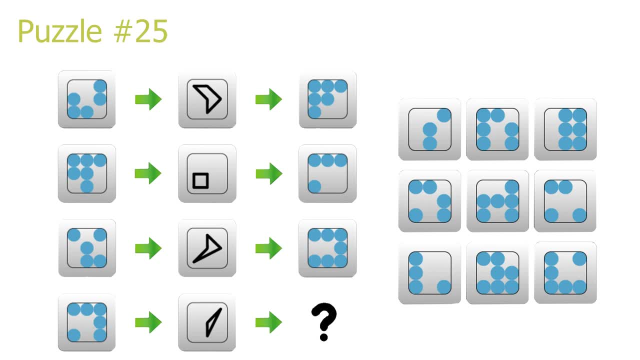 Puzzle 25.. This is a very interesting addition puzzle with cancellation. The polygon pictures in the second column represent a picture similar to the picture in the first column. The edges of the polygon are each a blue circle like this. Now to solve the puzzle, we just follow the rules. 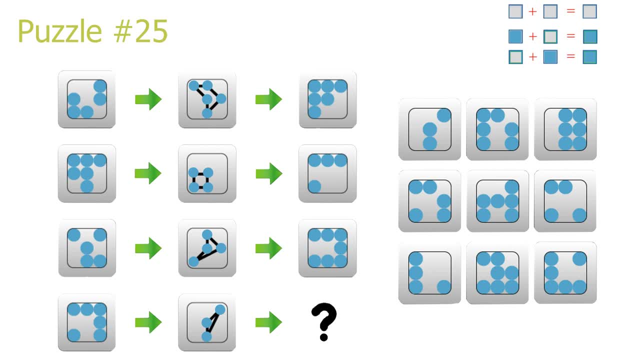 No circle plus no circle equals no circle. Circle plus no circle or no circle plus circle equals circle, And circle plus circle equals no circle. No circle plus no circle equals no circle, And so on. If we follow this addition for the fourth row, we get answer 8 as the correct solution. 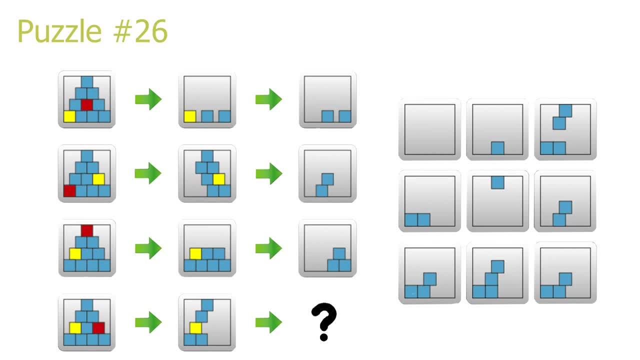 Puzzle 26.. This was another puzzle that I enjoyed very much. The best way to explain it is through the first row. Looking at the first picture in the first row, the red box explodes and destroys itself and every box it touches. The box floating in the middle of the air falls down to the ground. 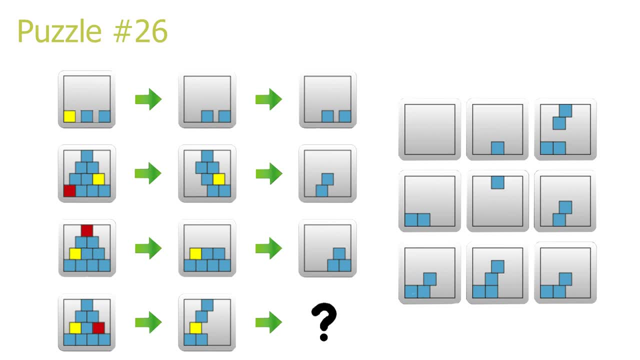 The exact same thing happens in the second picture. The yellow box explodes and destroys itself and every box it touches. It's important to see that it's not in direct contact with the box in the middle. If you're able to see it, you can see that the yellow box explodes and destroys itself. 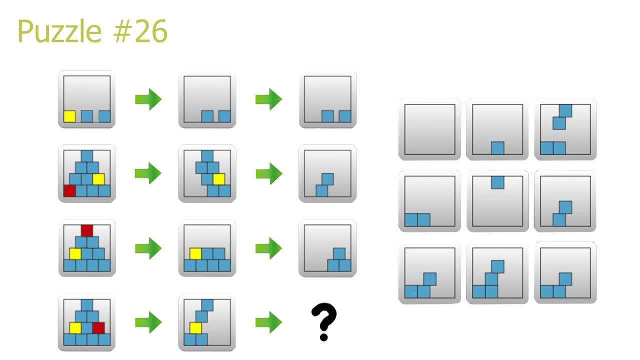 and every box it touches middle, even though they're very close. To solve the puzzle, let's look at the second picture in the fourth row. The yellow box explodes and destroys itself and the boxes around it. The box floating in the middle of the air falls down to the ground. Answer 2 is the correct solution. 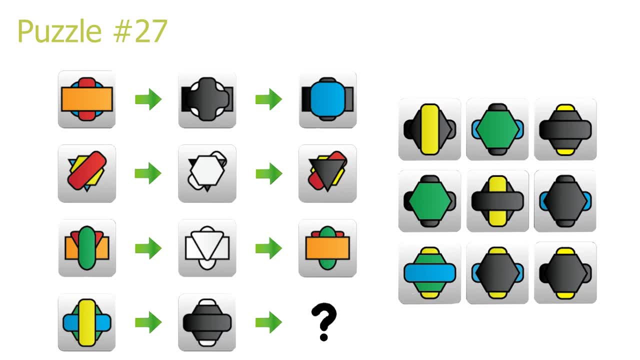 Puzzle 27.. In this puzzle we have three shapes stacked on top of each other. We are looking down on the stack of shapes from above. When we move to the right in the row, we take the top shape and place it on the bottom of the stack. There is also a color component to this puzzle. If our 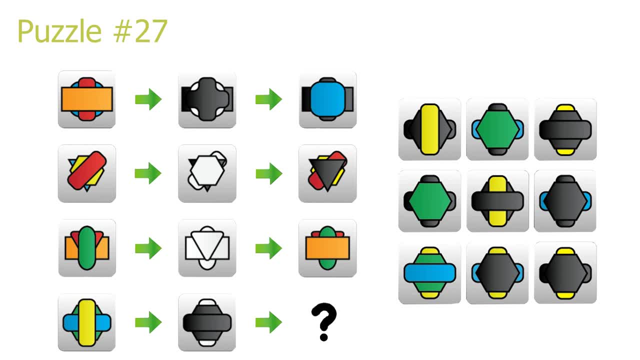 shape is black in the second picture in the row, then it's black in the third picture as well, And if our shape is white in the second picture, then the color of the shape in the third picture will be the same color of the shape in the first picture. To solve the puzzle, we look at the 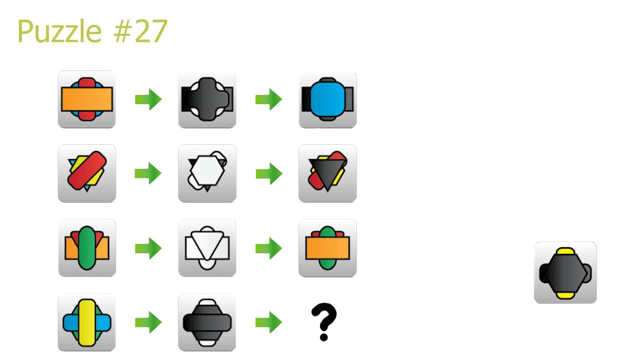 fourth row, We can tell that the horizontal shape and the hexagon shape will both be black, while the vertical line will be yellow. The vertical shape will be on the bottom, the horizontal shape will be in the middle and the hexagon will be on top. 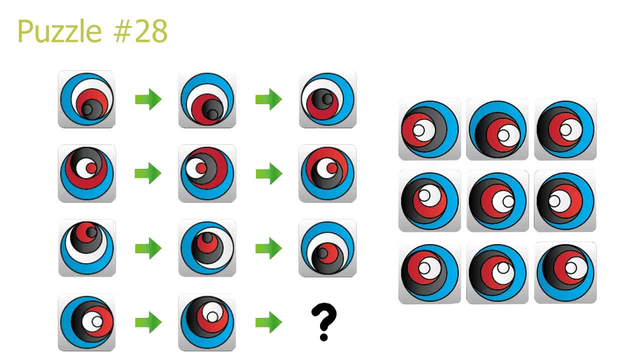 Answer 9 is the correct solution: Puzzle 28.. The hardest thing about this puzzle is keeping track of everything And making sure that you don't make an error. Basically, each circle move in some direction within the other circles and we have to keep track of what direction they're moving. 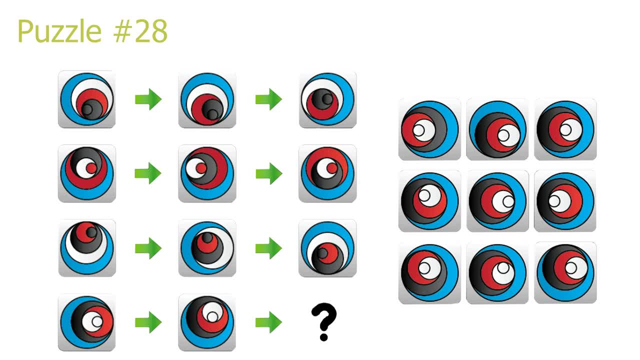 The key is to focus at one circle at a time. I'll use the first row as an example. Focusing on the white circle, we can see that it moves in a clockwise pattern. Focusing on the red circle, we can see that it stays on the bottom at all time. 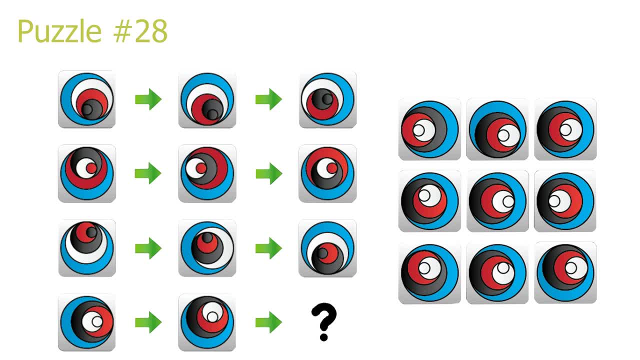 Focusing on the grey circle, we see that it moves in a counterclockwise pattern. To solve the puzzle, let's do the same thing for the fourth row. The grey circle moves in a counterclockwise direction and will be on the left side in the correct answer. 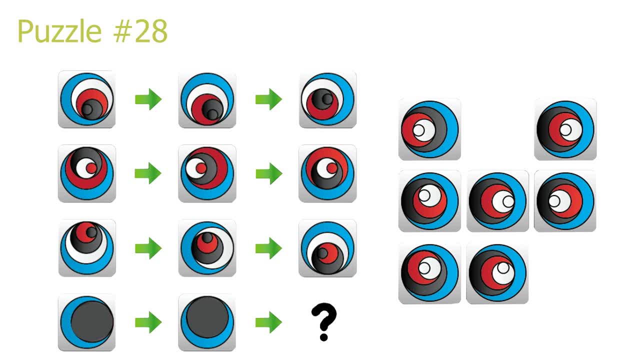 This removes answer 2 and answer 9 as possible. correct answers. Focusing on the red circle, we see that it stays on the right side at all time. This removes answer 1 and answer 7 as a possibility. Focusing on the white circle, we see that it moves in a clockwise. 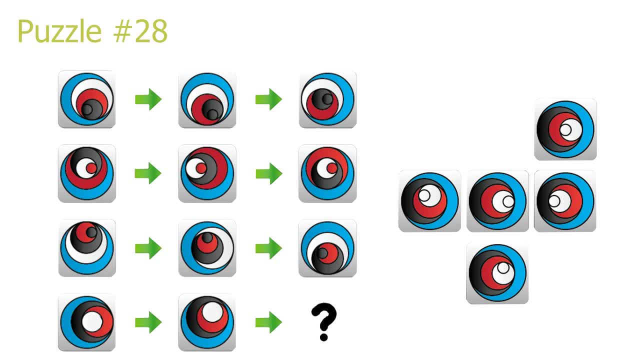 pattern and will be on the right side in the correct answer. This removes answer 4 and answer 6 as a possibility. Finally, the smallest circle also moves in a clockwise pattern and will be on the left side in the correct answer. This removes answer 5 and answer 8 as an option, leaving answer 3 as the correct solution. 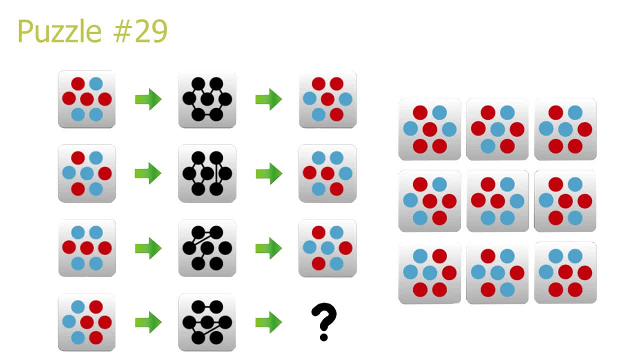 Puzzle number 29.. This is another very fun puzzle. In the second column we have this network of dots which describe how the circles move, going from the first to the third picture in a row, Going from the first to the third picture. the dots always move in a clockwise pattern within the network there inside. 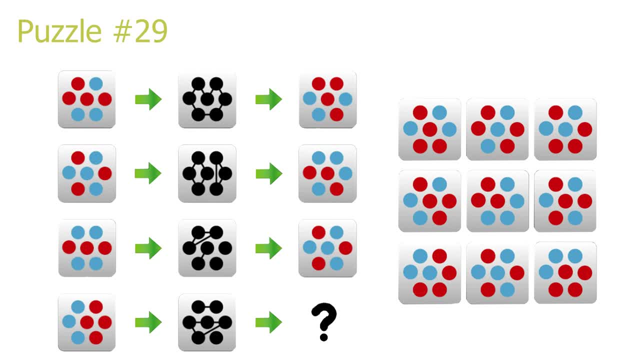 To solve the puzzle, we go by the fourth row. Looking at the second picture, we have three networks. We have two dots on top. These two dots will swap places. We have one dot on the bottom right, which will remain the same color, and we have four. 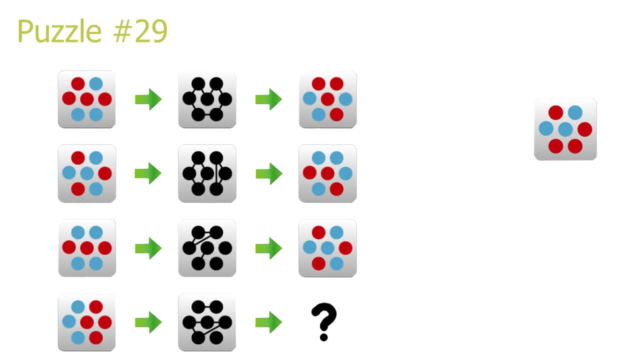 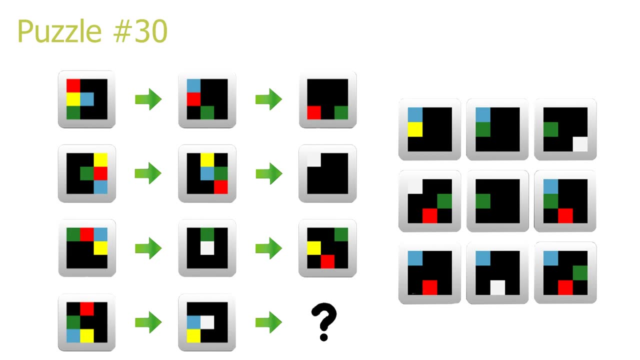 dots in the middle which will move in a clockwise pattern. This leaves answer 3 as the correct solution. Puzzle number 30.. In this puzzle we have these colored squares and a black background. The pattern of the colored squares is like this: 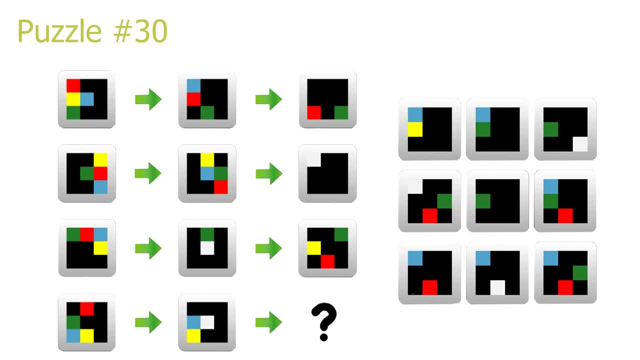 Moving to the right in a row, we can see that the colored squares move in a specific direction, one tile at a time. For example, if we look at the first picture, in the first row we have four colored squares. Going to the second picture, we see that the red square moves downwards. 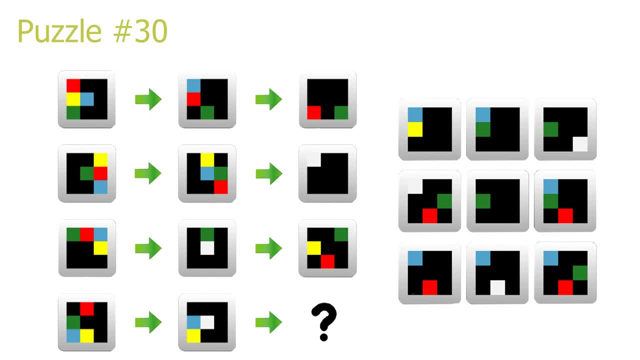 the blue square moves down, moves towards the top left, the green square moves towards the right and the yellow square moves outside the picture. Now notice that the movement I described for the red, blue and green dot remains the same, going from the second to the third picture. 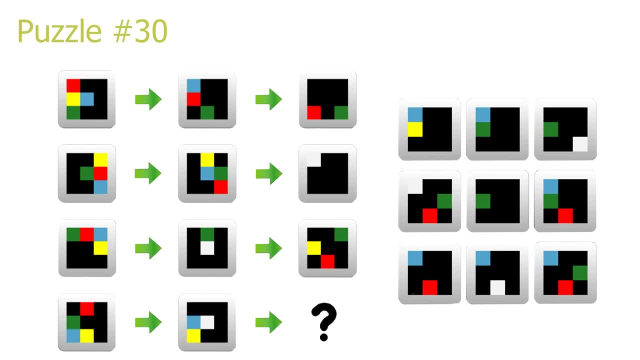 If we look at the three next rows, we see this new thing, which is this white square. A white square is simply two or more colored squares in the same position. To solve the puzzle, let's look at the fourth row. The yellow square moves towards the left and will leave the frame going from the second. 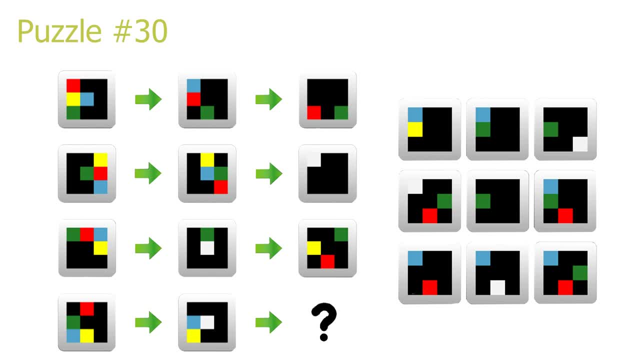 to the third picture. The blue square moves upwards and will end up in the top left corner in the third picture, Because there is only the red and the green square left. we know that they are both inside the white square, So the red square moves downwards and will end up in the middle bottom in the third picture. 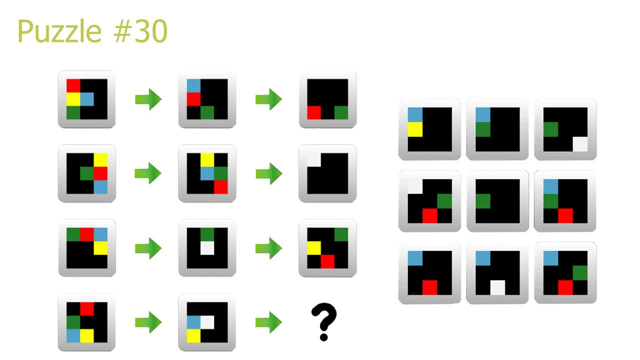 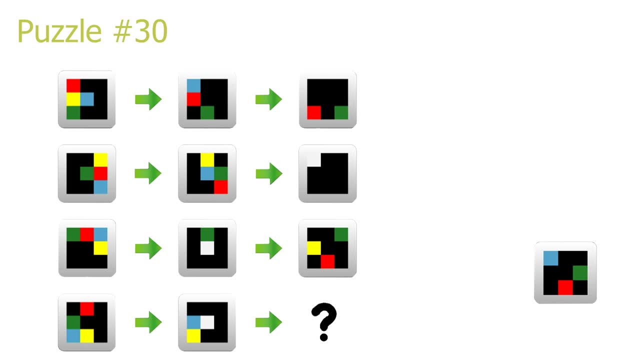 The green square moves towards the right and will end up in the middle right. in the third picture, The blue square is in the top left, the green square is in the middle right and the red square is in the middle bottom. Answer 9 is the correct solution. 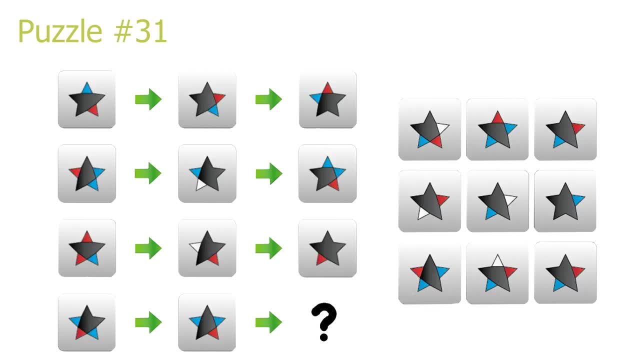 Puzzle 31.. This was the first puzzle I found an error in. If we look at the first row, we can see that the puzzle is moving to the right. in the row, The red corner moves in one position in counterclockwise direction, while the blue corner moves in two. 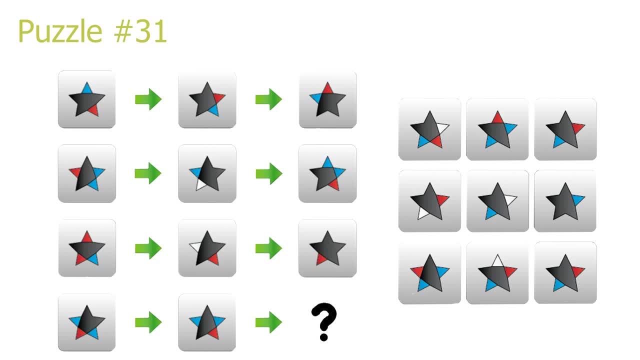 positions in clockwise direction. Looking at the second row, we can see that a white corner is produced when a red and a blue corner overlap. If we look at the third row, in the second picture we have a white corner and a red corner, But going from the second to the third picture, the white corner disappears. 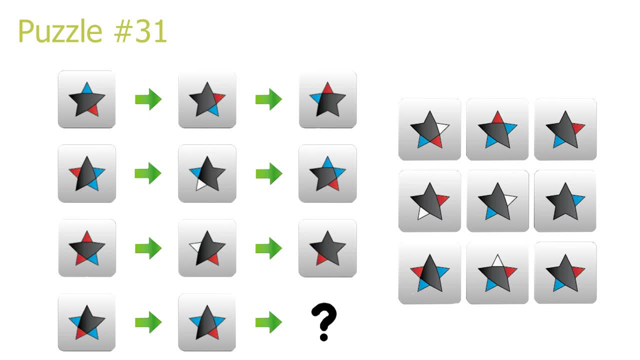 I think this is just a design flaw from the puzzle creator. To solve the puzzle, we look at the second picture in the fourth row. Moving the two blue corners in two positions In clockwise direction leads to a blue corner in the bottom left and the top right. 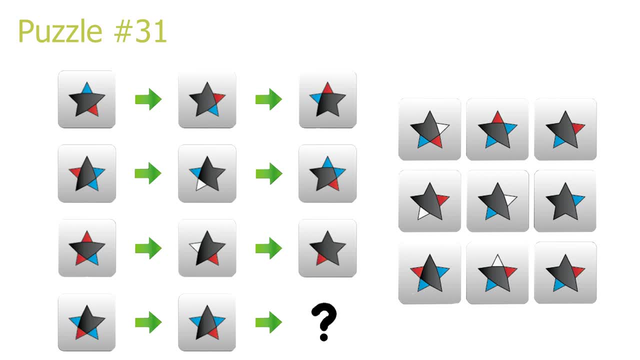 Moving the red corner in one position in counterclockwise direction leads to a red corner in the top right. Because we have a blue and a red corner in the top right, it will turn white. The answer will have a blue corner in the bottom left and a white corner in the top. 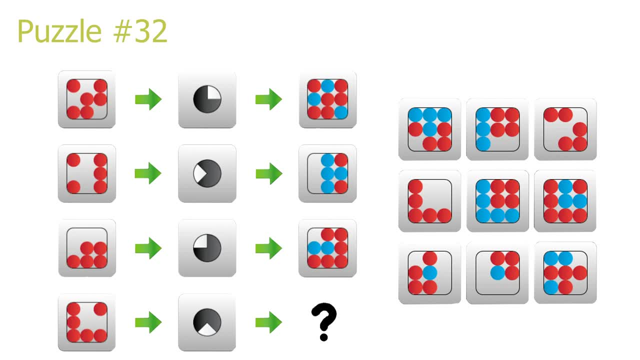 right Answer. 5 is the correct solution: Puzzle 32.. This might be the most difficult IQ test puzzle that I've ever come across. After around 2 hours of trying to solve it, I gave up and asked for help. I'll be very impressed if any one of you watching is able to solve it by yourself. 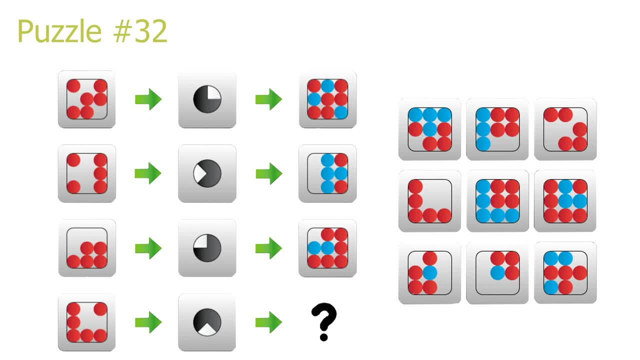 I don't want to ruin the puzzle for anyone who wants a challenge, so before giving the correct answer, I will give it 3 hints. Pause the video now if you don't want the first hint. Ok, Hint number 1.. If we give the red circles a value of 1 and the blue circles a value of 2, then the total: 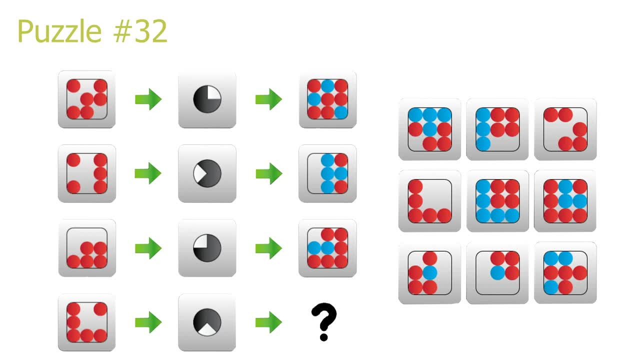 value in the third picture will always be double of the total value in the first picture. For example, in the first row we have 6 red circles. in the first picture this gives a value of 6.. the first picture and in the third picture we have 6 red circles and 3 blue circles. 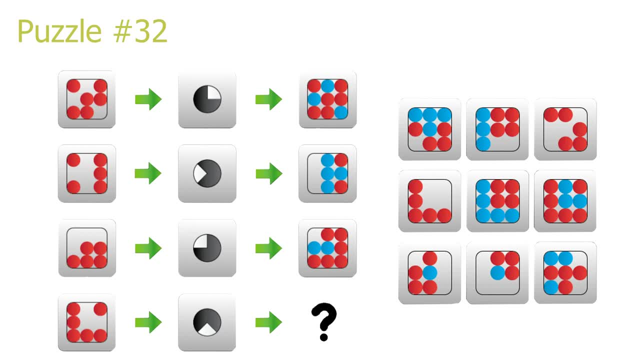 This gives a total value of 12 in the third picture. So because the value is 6 in the first picture, it will be 12 in the third picture. Pause the video now if you don't want the second hint. The second hint is that when I look at the second column I see these knobs on the oven. 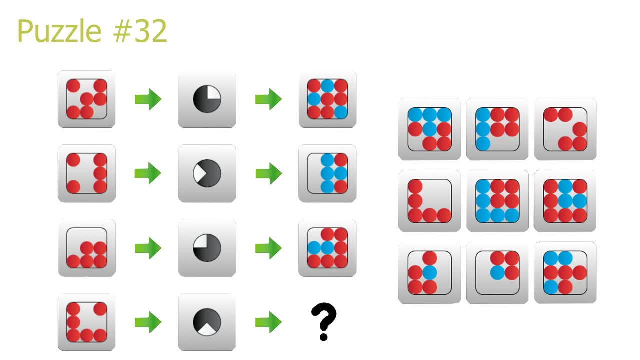 which you rotate to change the temperature. Because of this, I assumed that the puzzle had something to do with rotations. Instead, you should view the second column as these arrows which point from the center and outwards in the line where black and white meets. 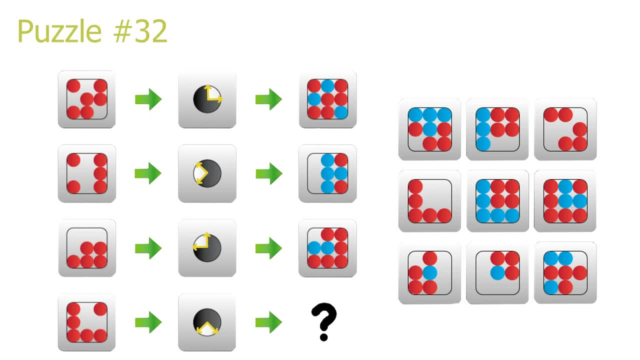 Pause the video now if you don't want the third hint. The third hint is that the puzzle is a form of an addition puzzle and adding two red circles together gives a blue circle. That was all the hints. hopefully some of you took the hints and was able to solve the. 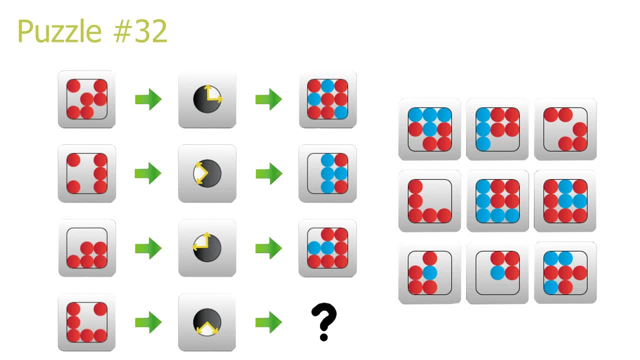 puzzle by yourself. I will use the first row as an example for how the puzzle works. Let's start by removing the rest of the rows to have some space. We take the first picture And we take one of the arrows. This indicates that we should move all the circles up by one. 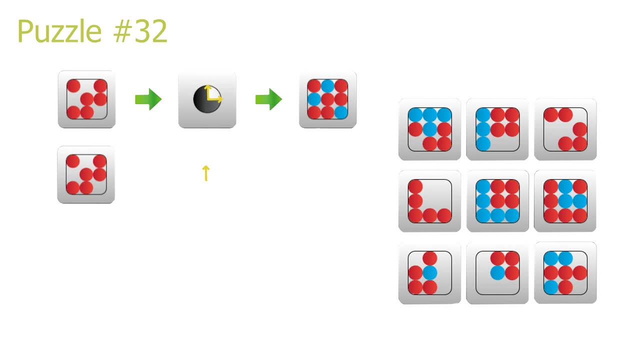 The circles which fall outside the picture on the top reappear on the bottom. This produces this picture Again, we take the first picture and we add the second arrow. This indicates that we should move all the circles to the right by one, Which produces this picture. 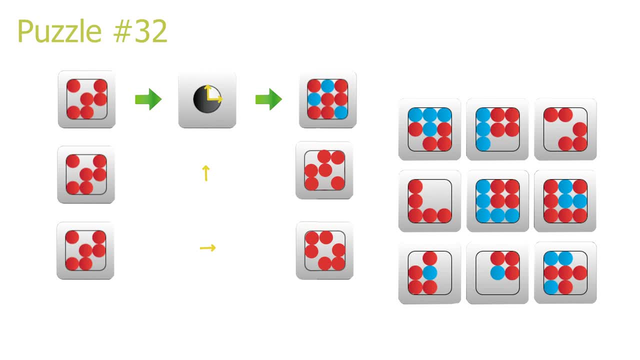 Now all you do is simply add these two pictures together to get the third picture. Two red dots become a blue dot. Now that you understand the method, let's solve the puzzle Again. let's remove everything but the fourth row. We take the first picture and one of the arrows and move everything towards the bottom right. 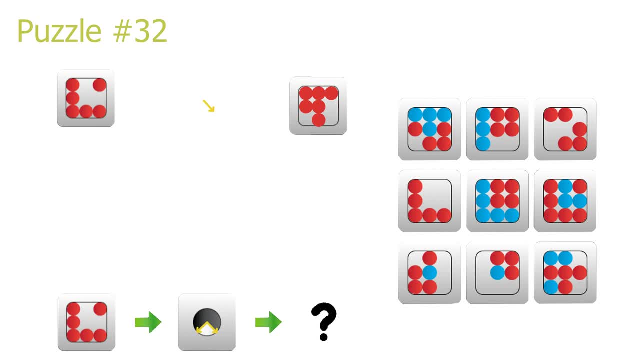 Moving towards the bottom right is the same as moving once towards the right and once downwards. Again, we take the first picture and we add the second arrow and move everything towards the bottom left. Now we have these two pictures and we add them together to get answer 1 as the correct. 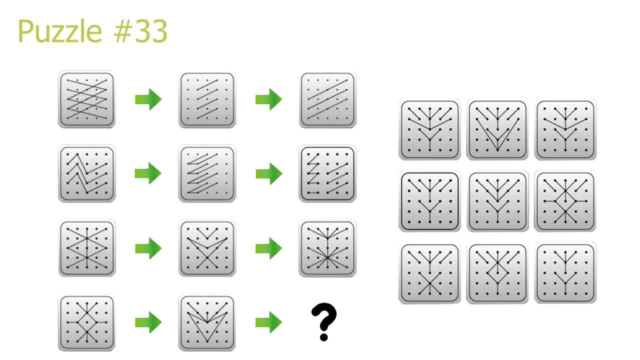 solution: Puzzle 33.. This is a very well designed puzzle. In this puzzle we have these lines which are connected to the dots, and we added the two first pictures in a row to produce the third picture. If the path of two lines cross, then they cancel out. 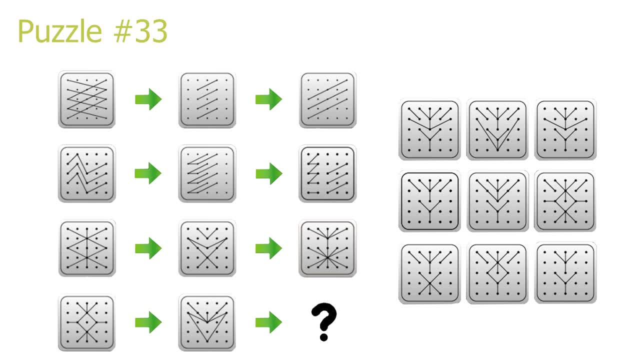 Let's use the first row as an example. In the second picture we have lines between these dots. Let's start by moving them over to the first picture and then adding lines between them. We can clearly see how the lines in the second picture cut, every line going from the top. 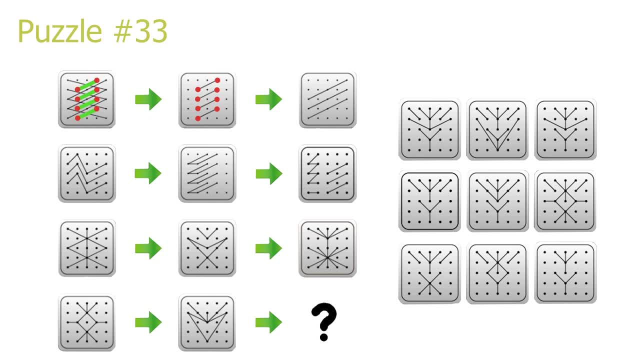 left to the bottom right. This leaves three lines, which goes from the top right to the bottom left, which we can see in the third picture. There is one more important detail to solve the puzzle, Puzzle 34.. In the third row we have a new situation. 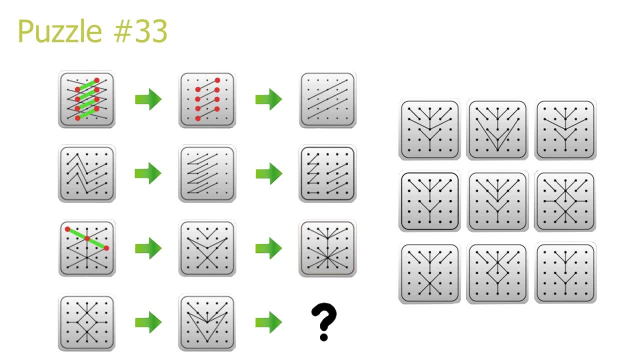 In the first picture we have three dots in a line like this. Now, is this a singular big line or two small lines? This question is important because we don't know what happens when we cut the line. Looking at the second picture, we have these two points and a line between them. 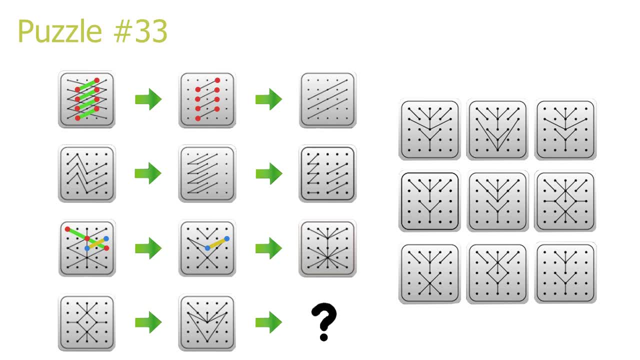 Adding them over to the first picture, we see that it cuts the line which I previously talked about. Now, looking at the third picture, we see that the top portion of the line is conserved and therefore we know that it's two small lines and not a singular big one. 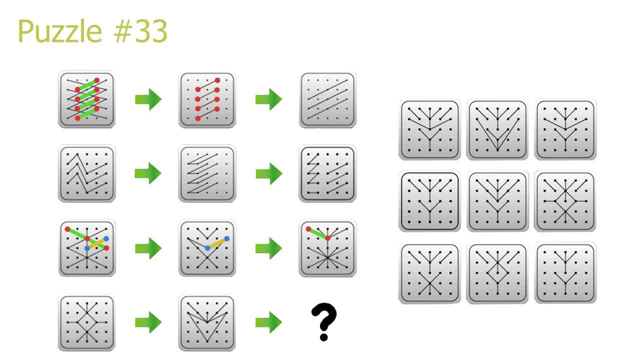 Puzzle 35.. In the third picture we have three dots in a line like this and they are quite easy to find. The first rule is that if a line goes through two or more lines, then all the lines are cut. We can see this in the second row. 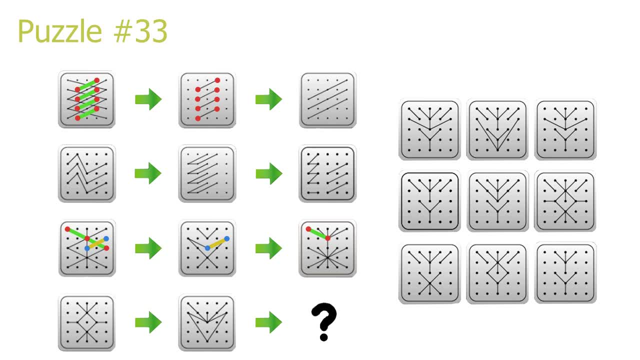 The second rule is that if two lines extend from the same point, then they do not cut each other. To solve the puzzle, let's go by the fourth row. In the first picture we have these dots and these lines connected to them. Adding them over to the second picture, we can see which lines get cut. 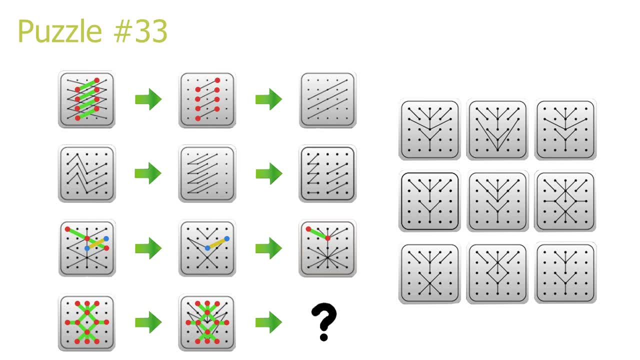 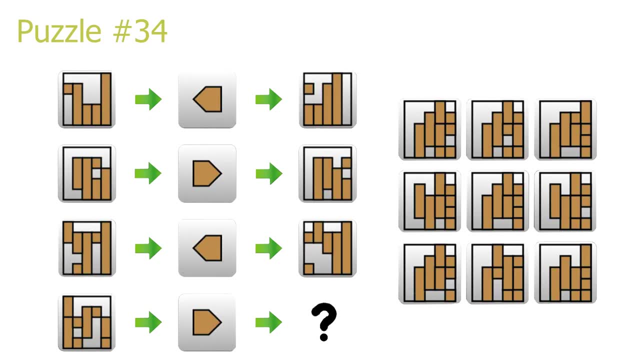 Pause the video if you want some time to look at it. But basically, after our early cutting, we are left with this picture, Puzzle 36.. In this puzzle we have these arrows in the second column which point towards the left or towards the right. 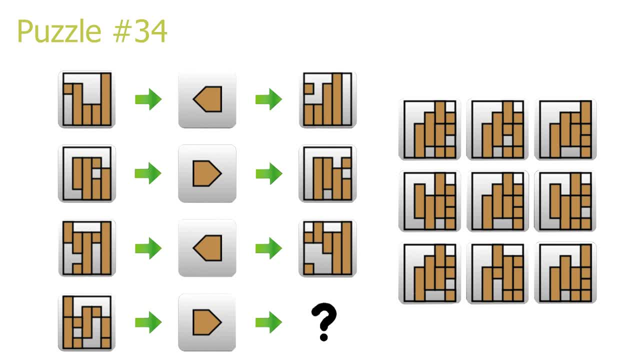 The shapes in the first picture are organized from smallest to biggest in the direction of the arrows to produce the third picture. I will go through all the incorrect answers and why they are incorrect. Answer number 9 has this box which are marked in blue and if we look at the first picture, 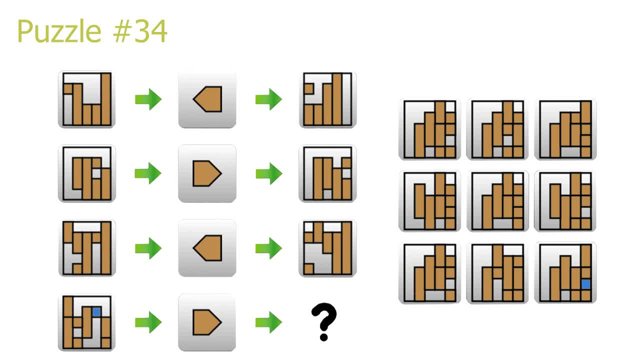 in the fourth row. we have this fourth box in this position instead, so answer 9 is not correct. This box is in the wrong vertical place. Next, I want you to look at answer 2, answer 3 and answer 8.. They all have a smaller box on top of a bigger box. 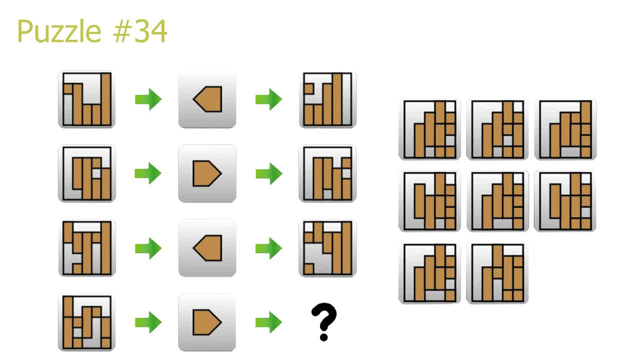 This breaks the rule of always sorting from smallest to biggest in the direction of the arrow. Therefore, these answers are wrong. Next look at answer 4, answer 5 and answer 7.. They all have the small boxes in the wrong position. This leaves either answer 1 or answer 6 as correct. 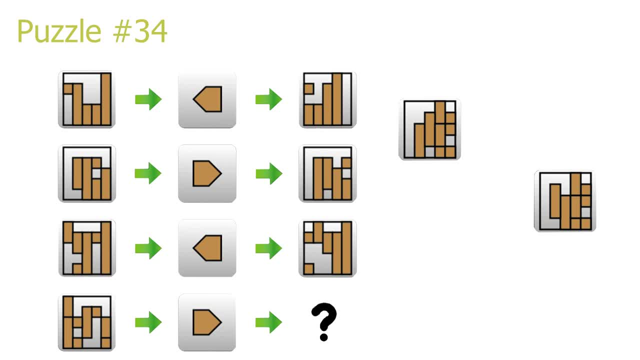 The only difference between these two answers are the biggest rectangles. If you look at the first picture, you can see that the first box is in the wrong vertical position. If you look at the first picture, in the fourth row, the two rectangles are placed like this: 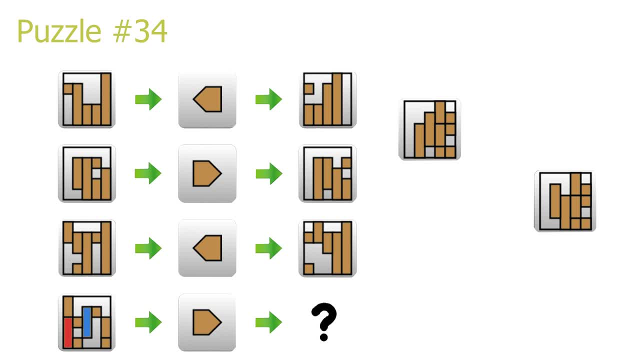 The red rectangle is on top and the blue is on bottom. Looking at answer 4, we know it can't be correct because it has blue on top and red on bottom. Answer 1 is the correct solution. Puzzle 35.. I have not found a simple solution to explain the officially correct answer. 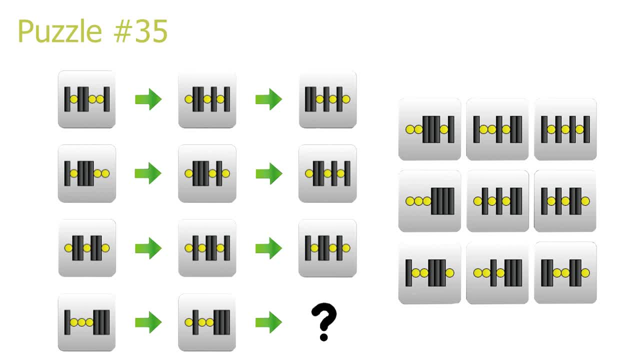 I would really appreciate any comment explaining this puzzle in a simple way. So let's go through how I solved the puzzle and how I came up with a wrong answer. The first priority of the puzzle is to separate an equation. The first priority of the puzzle is to separate any two dots connected. 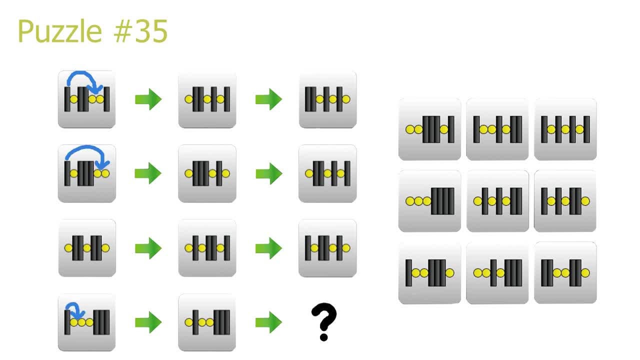 We can see this in the first row, second row and fourth row. Notice that it's always the most left bar which is placed between the dots. After this is fulfilled, the next thing to do is to move the leftmost object to the rightmost. 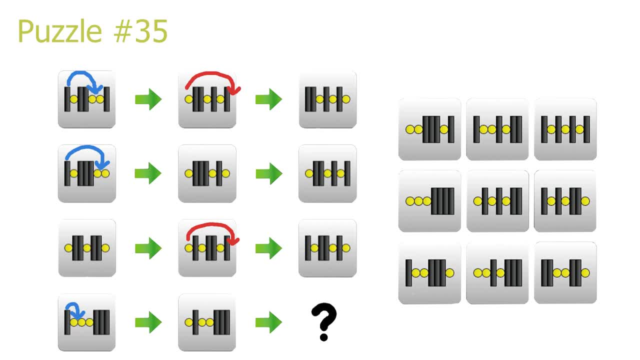 position. We can see this in the first row and the third row. Now you would expect the puzzle to move the leftmost object to the rightmost position in the second picture in the second row, But the problem is that this would create a pair of dots right next to each other, which 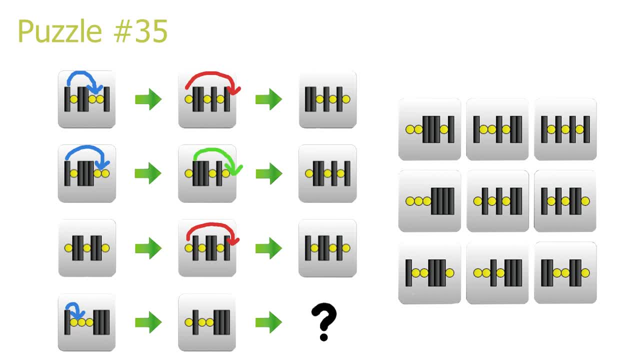 would break our first priority, Puzzle 36.. We move the leftmost bar to the rightmost position. We can also observe this in the first picture in the third row. To solve the puzzle, we look at the second picture in the fourth row. 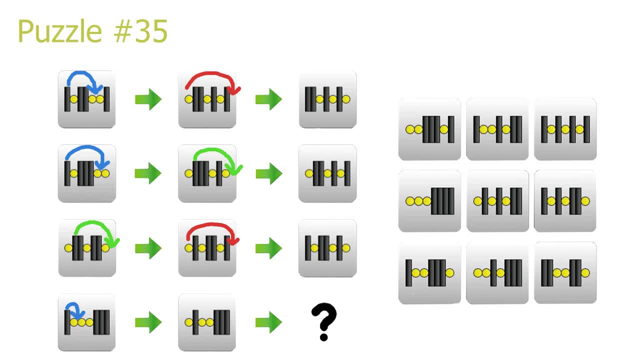 Notice that we have a pair of dots right next to each other and we have to use the leftmost bar to place it between them. The problem is that moving the leftmost bar would create a new pair of dots right next to each other and therefore we use the second, most left bar.